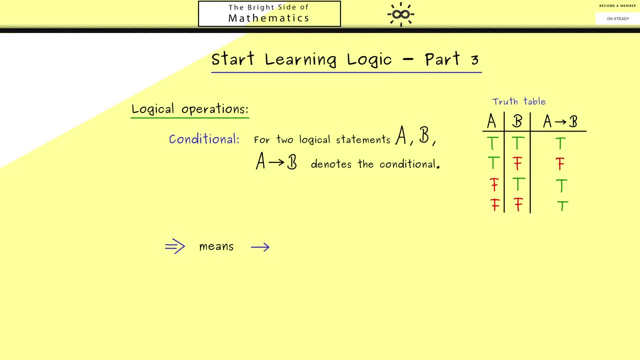 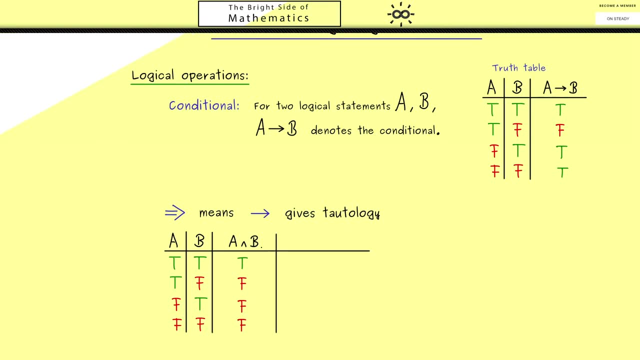 that the normal error, the conditional gives a tautology. If this seems confusing, the next example will definitely help. Okay, here you see a truth table where we have a and b and a conjunction. And now i want to look at this conditional where you see the conjunction binds closer. 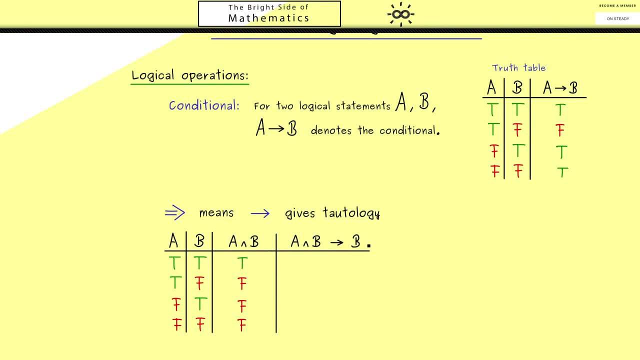 than the conditional error. Therefore we don't need any parentheses here. So now, by the definition of the conditional, we go from true to true, So we know this one is true. but then we go from false to something, So we know all the other ones are also true. So we have proven that this 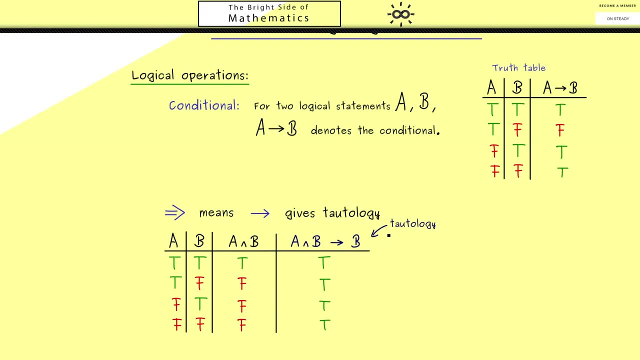 combination which gives us a logical statement is indeed a tautology. Therefore we can write: and b logically implies b. So you see, this one i actually call implication and it is almost the normal conditional, just with an extra bit of information. Now we are already going into the 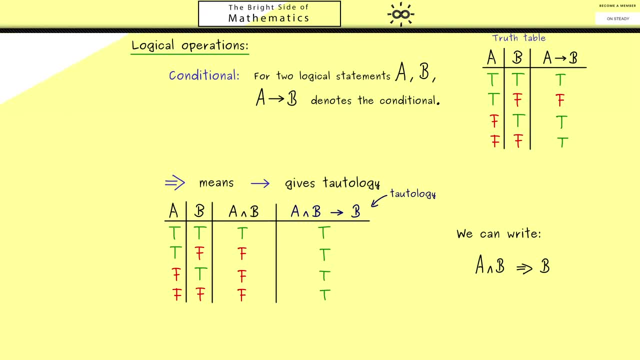 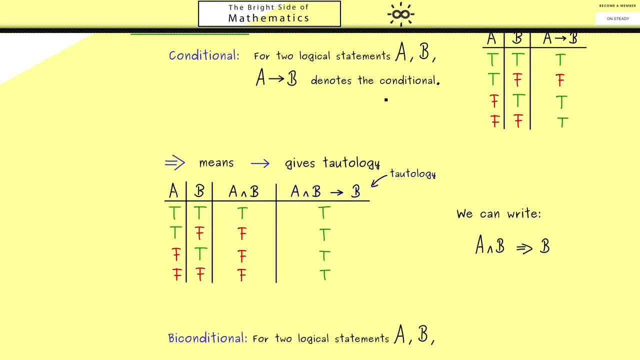 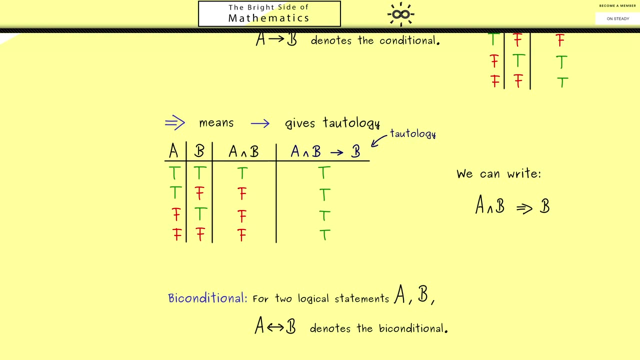 direction of deduction rules and proofs. but before we do that, i first want to show you one last logical operation. It's the so-called biconditional and, as the name suggests, it's the normal conditional in both directions. Therefore, the notation is just an arrow pointing in both directions. 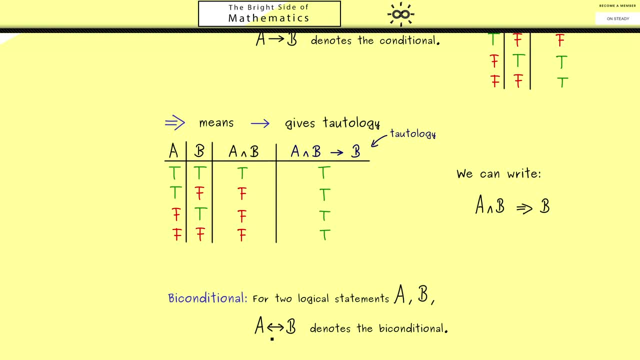 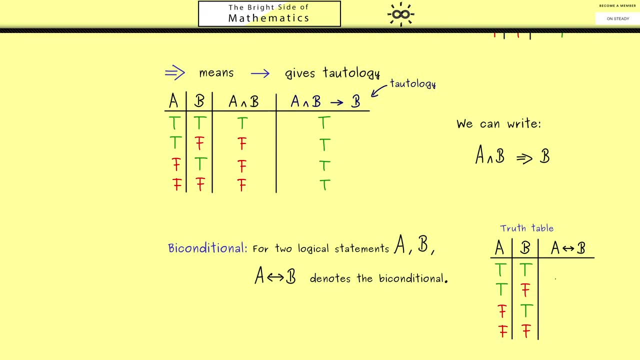 and we would read that as a if and only if, b. As before. i give you the definition by writing down the corresponding truth table. Now, if and only if should of course mean that the truth values on both sides should coincide. So here we have true. In the same way we have true in the last line. 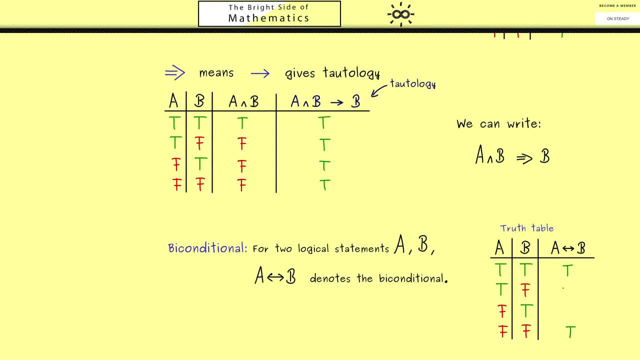 because we have false on both sides. However, in the middle it's mixed. therefore, if- and only if- should give you here a false, Most of the time, you will be interested in the case that the biconditional is true, which means the truth values on both sides coincide. Therefore, this perfectly fits with. 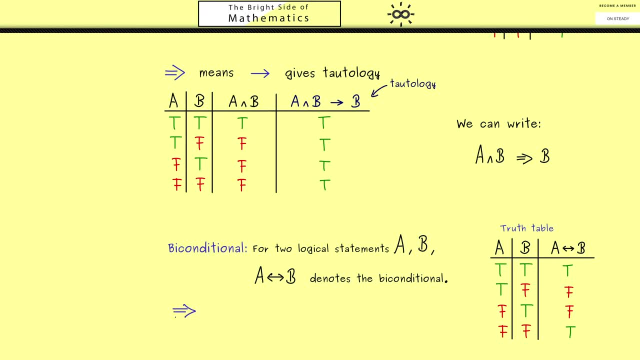 the notation we already used for the logical equivalence, because now it's the same as saying that the biconditional gives us a tautology. Now, if you think that's all confusing, then maybe the next table will be clear. Now let's run this again. 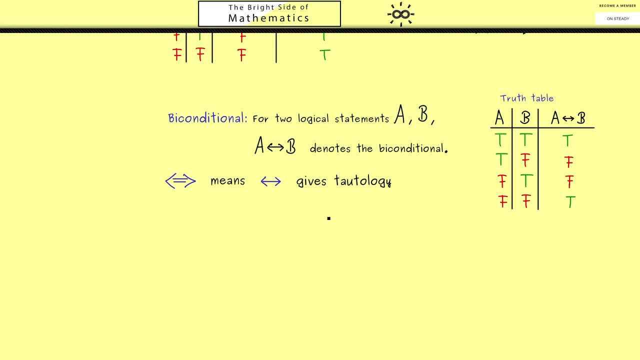 example makes it even worse, but then it's a good exercise for you. Please try showing, by using a truth table, that a, if and only if b is logically equivalent to the conditional a b and the conditional b a. Of course, this is what we wanted. 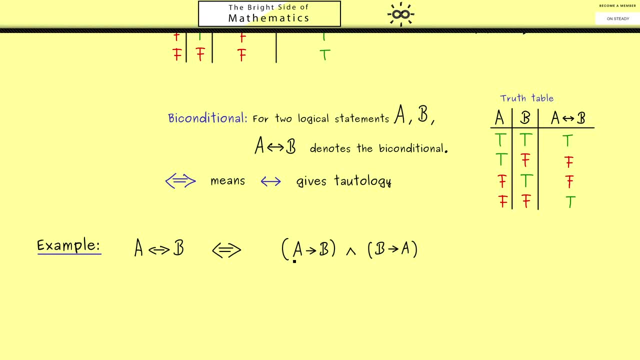 from the beginning that the biconditional is just a normal conditional in both directions. Now you can still practice working with truth tables with another example, which is also very important. It's given by: if a, then b is logically equivalent to: if not b, then not a. Now this is known as the 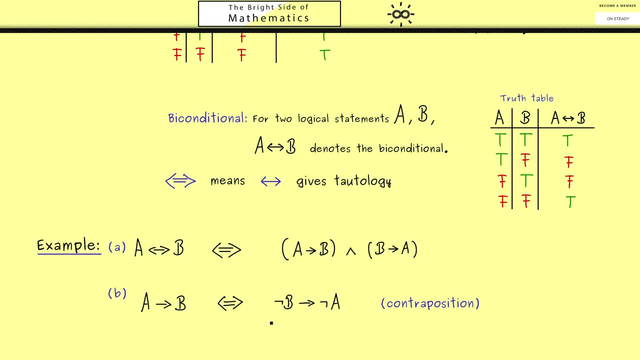 counter position. You can change the order in the conditional, but then you have to add the negation sign on both sides. Now to get an idea or a visualization why this is logical, let's consider again an example. in the English language, There is fog, is our statement a, and we have poor visibility, is our statement b. 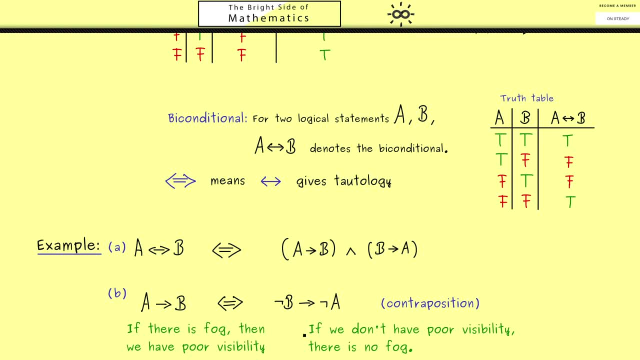 And then we have our if then statement here. On the other hand, not b would mean we don't have poor visibility, and not a would mean there is no fog. Now, if you read this, it makes sense and, of course, if you know, when we have a, then we have. 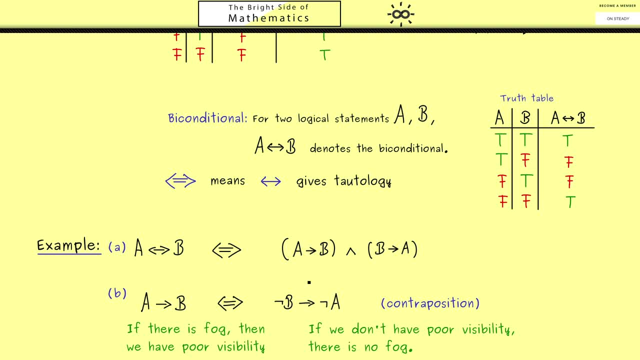 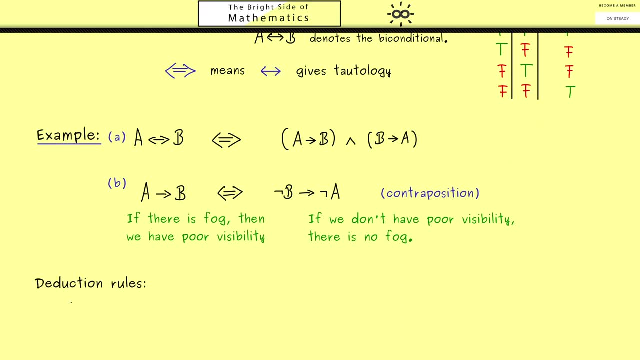 b, then you also know when we don't have b, we can't have a. With the counter position, we have a first example of a so-called deduction rule. Such a deduction rule basically tells us how we get new true logical statements out of known true logical statements. 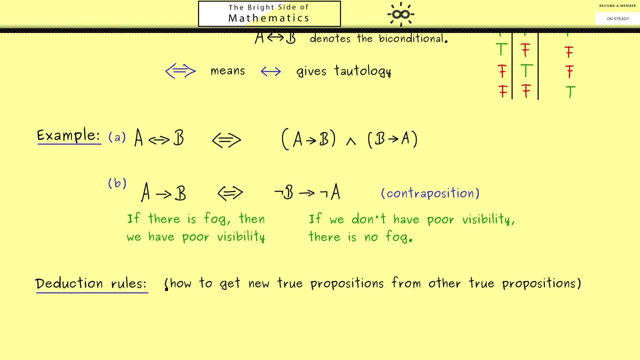 When we have the deduction rules- we don't never write down any truth tables any more, because we can just apply these rules- then Maybe the simplest one, and also the most important one, is Modus Ponensh. For this we have 2 premises. 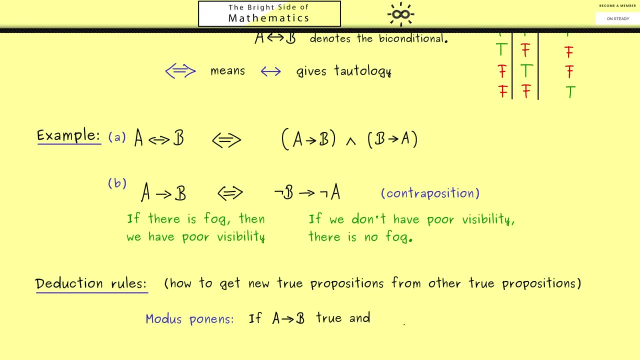 First we assume that a to b, First we assume that a to b, First we assume that a to b, b is true, and secondly we assume that a itself is true. Then the conclusion is that also b is a true logical statement. 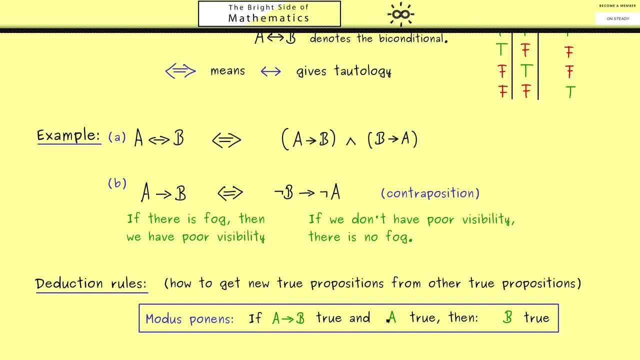 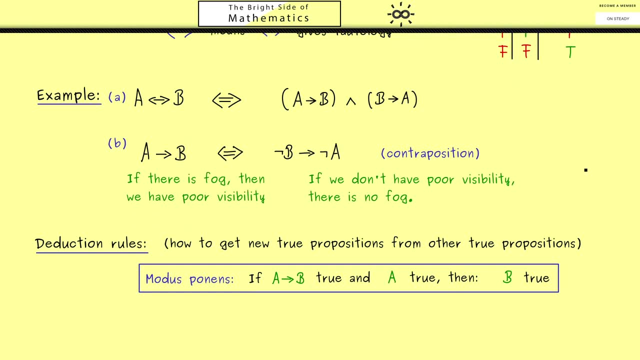 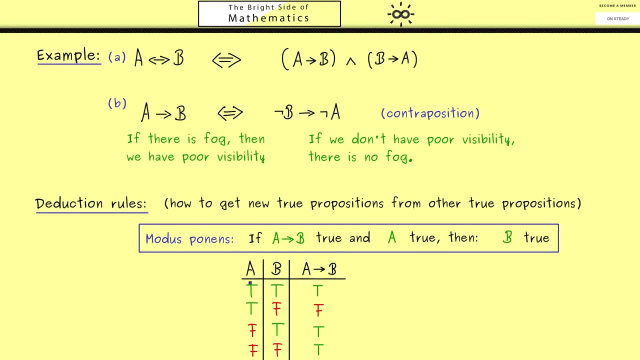 So you see, it's very simple. when you know that these two statements are true, then we get out a third true statement. So maybe for you it seems logical, but of course we can write down the proof by using a truth table. Now we don't need a new one, because we already have the one from the conditional and that's. 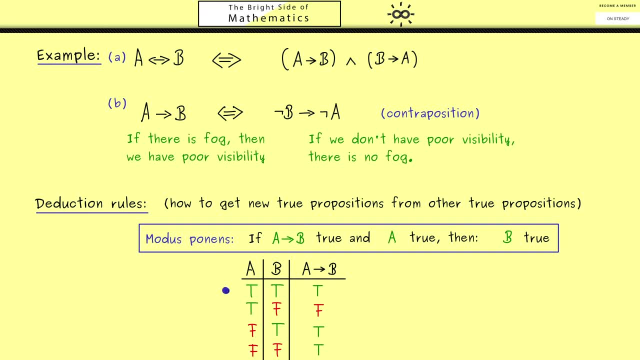 all we need here Now. since a has to be true, only the first two rows are interesting for us. On the other hand, the statement: if a, then b has to be true. so we have here the first line, the third line and the fourth line. 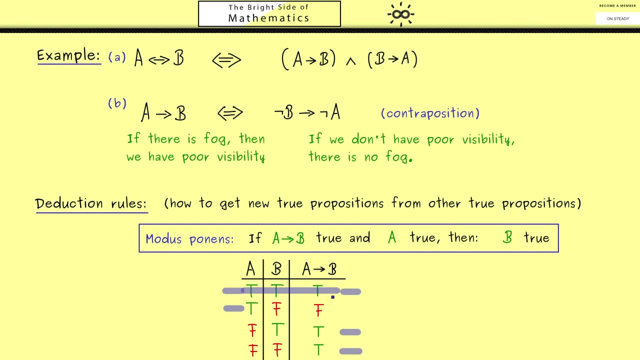 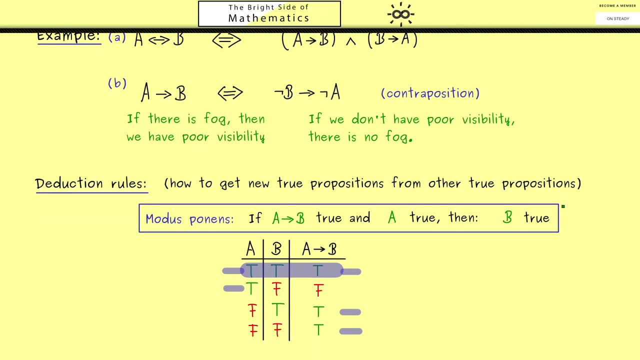 And there you see, the only intersection we have is the first row, And there we can just read the truth value for b: Ok, so this is a deduction rule we will apply later when we write down proofs. Another important one is the so called Shannon rule. 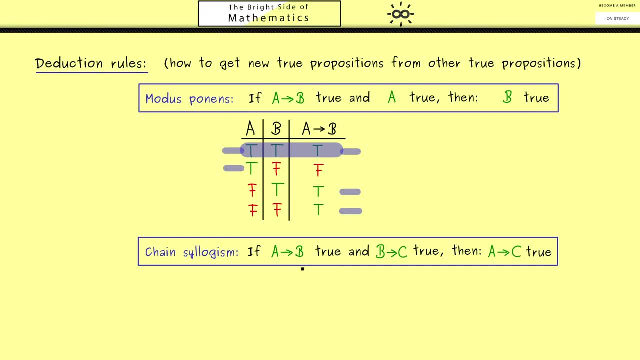 Shannon Syllogism. It simply tells you, when you have two conditionals where you know that they are true and that b is on the right hand side for the first one and on the left hand side for the second one, then you know that the conditional- if a, then c- is also a true one. 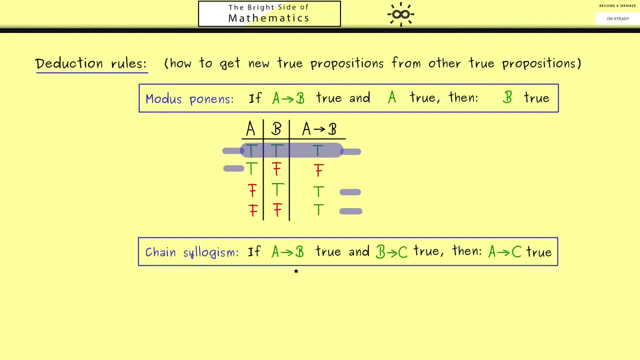 Of course, this is also very useful because in mathematics we often have implications, and this means you can put them into a chain and get out a new implication in the end. Ok, Now, the last deduction rule I want to show you today is a very popular one. 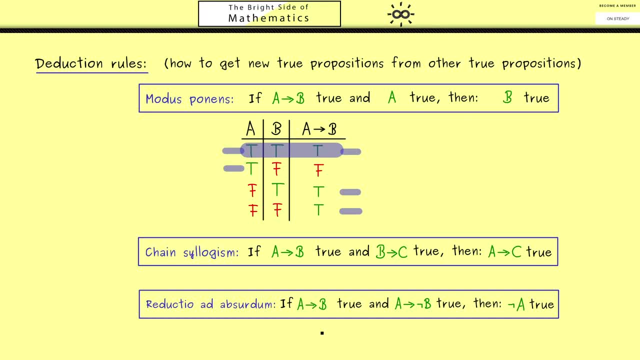 It's the reductio ad absurdum. This one describes a contradiction. so if you know that a implies b and a implies not b, so both conditionals should be true, then a would imply a contradiction. therefore it must be false, Or in other words, not a is then a true statement. 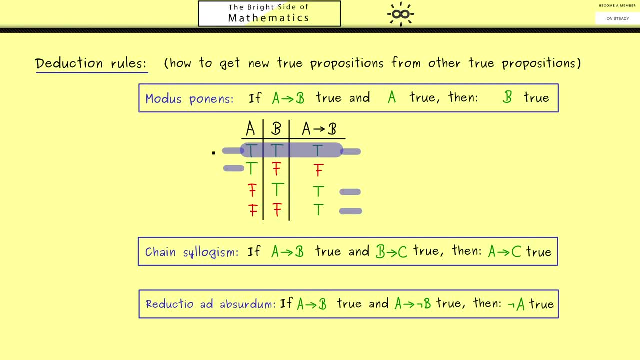 I think that's a good exercise for you, so please write down the truth table and check if that is indeed correct. Ok, that's enough logic for the moment. In the next videos, we first talk about sets and maps and then we put everything together.